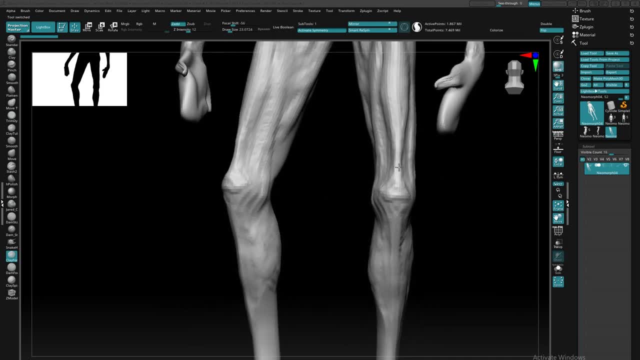 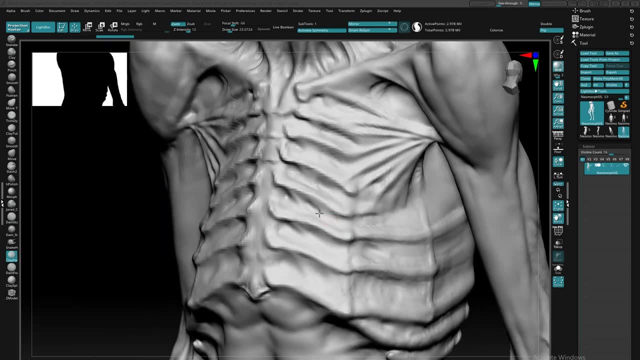 we can create a custom topology in something like Maya or another external 3D package, which tends to be not the most time efficient for what I'm trying to do at this point in my production process. The other choice is going to be using auto re-topology, which at this stage I don't need. 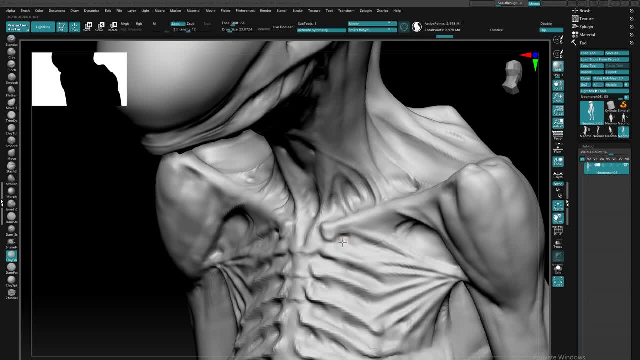 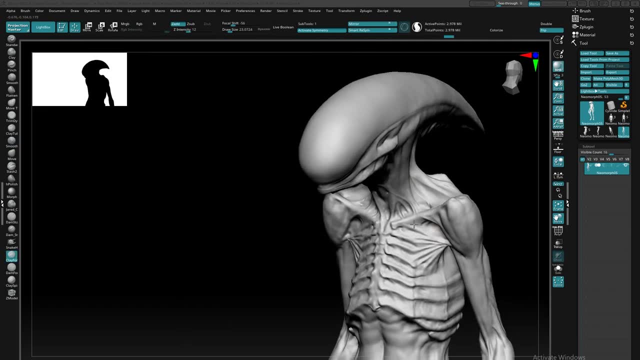 a hundred percent final geometry, but I want something that's easy to manipulate as well as has nice quadding to start sculpting on top of, Which Zremesher is the best way to get your topology to start sculpting on top of? Also, one thing that is nice to have at this point is a little bit more control. 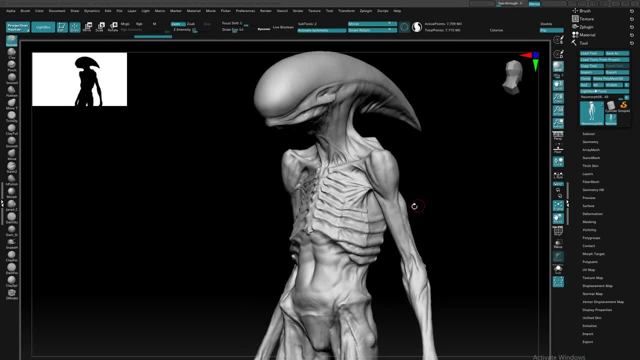 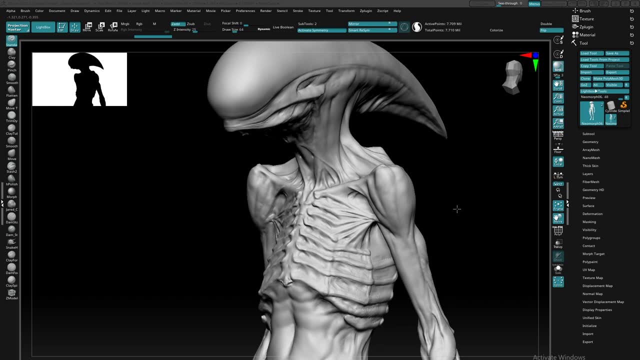 over where the poly rings end up, so I can create quicker selections and I don't have to worry quite as much about things like spirals that Zremesher can produce. So I'm going to go ahead and show you guys how I accomplish that control using Zremesher. So the first thing that I like to do, 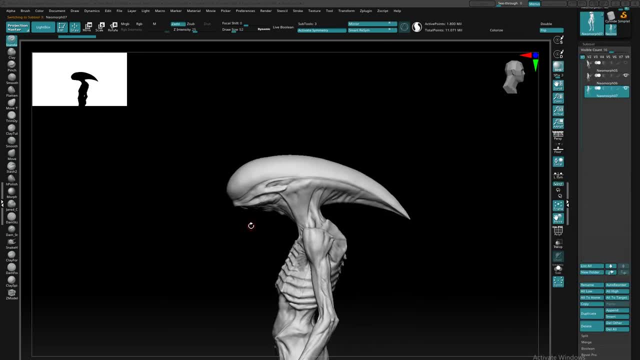 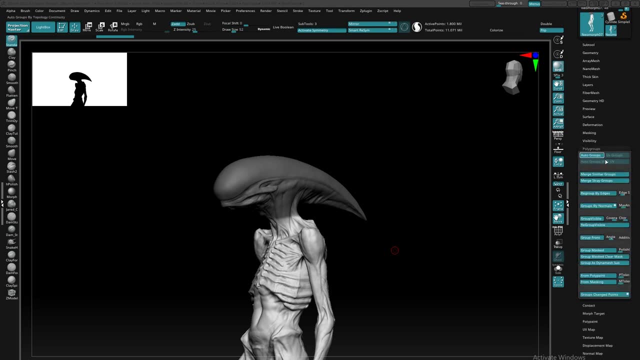 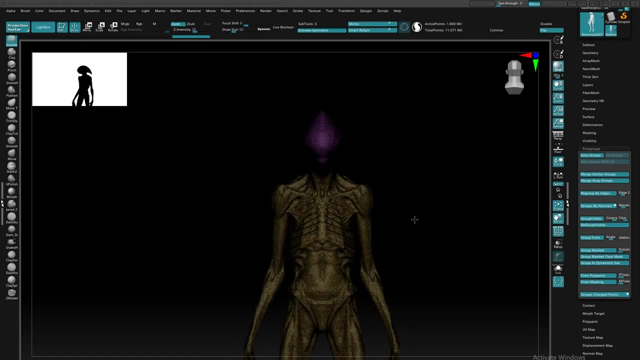 is using the mask lasso brush. I mask out where I want edge loop to occur, So I'll mask out the head. once I have that, I'm going to come down here to my polygroup menu and hit group by mask. This is going to create a polygroup that's going to tell Zremesher to make a clean edge around these. 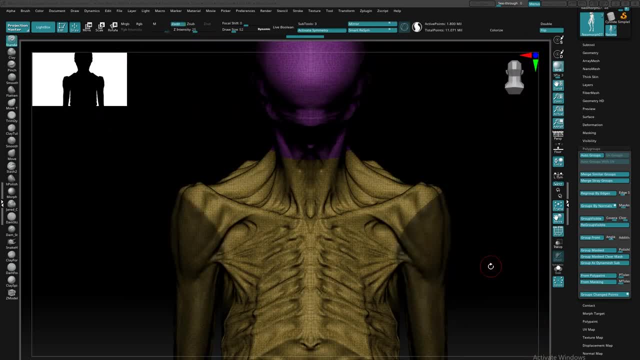 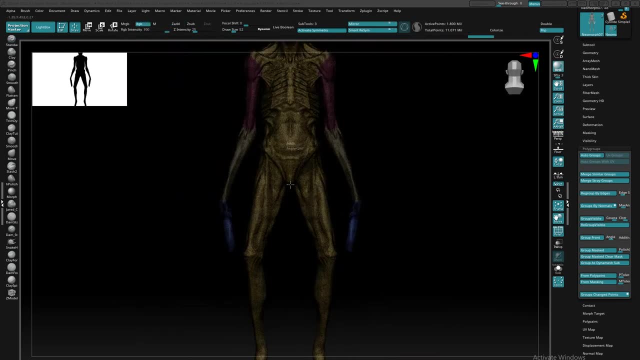 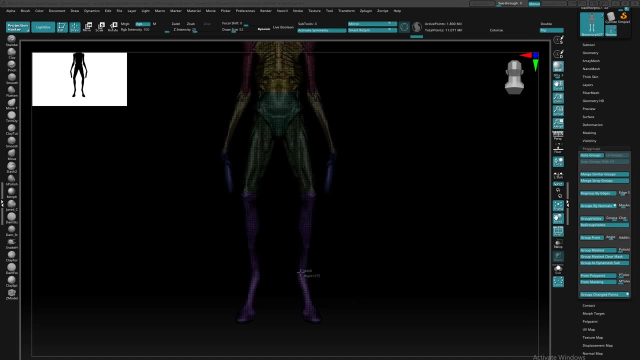 two points. So once I have that, I'm going to start throwing polygroups around the areas that I want loops to be at. I most likely tend to stick to areas that have things like joints, so shoulders, elbows, knees, hips or just any other areas where I want a nice clean loop at Once I've gone through. 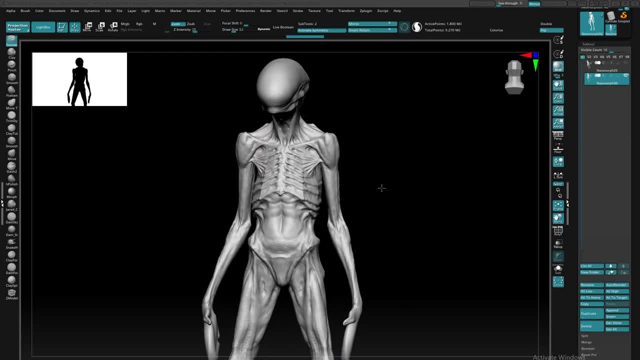 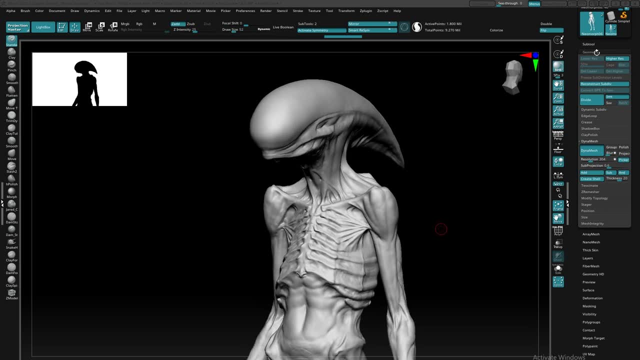 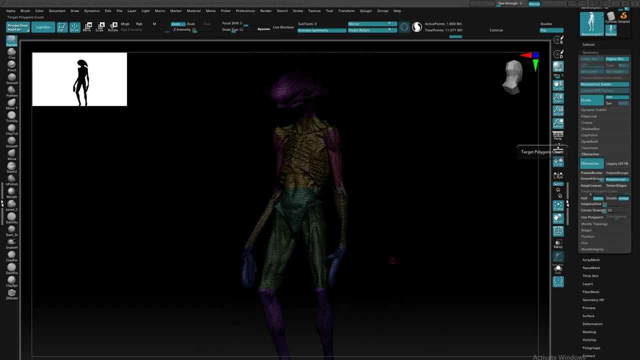 and established my polygroups. next I'm going to start running the Zremesher. For this part, I like to duplicate my original dynamesh so that I can re-project that model into my new quadded out mesh. So to do that, we'll come over here and select duplicate. Next, inside the Zremesh drop down, 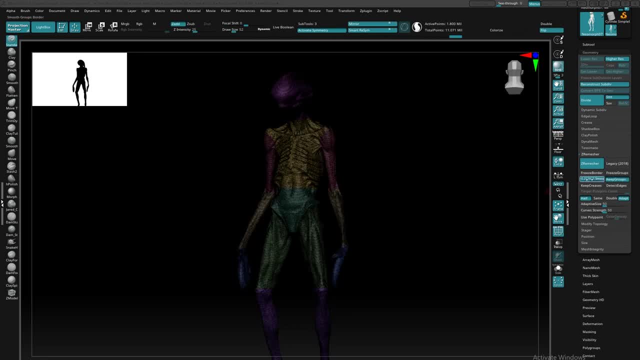 I set it to half and make sure that keep groups is checked and smooth groups is set to one. Then we'll hit Zremesh. Now we can see our clean topology, which is a little too dense, but we do have some of that edge control and areas around the polygroups, which is what I wanted. 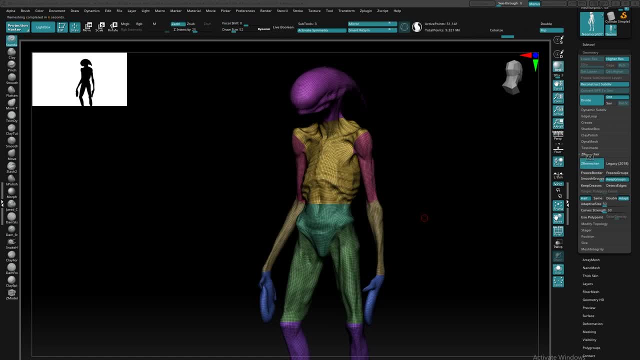 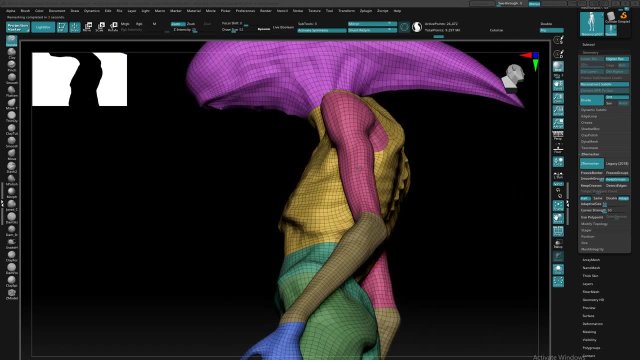 So let's just go ahead and hit Zremesh a couple more times to get something a little bit lower. Usually I'll take the mesh down as low as I can, while still keeping the shape of the model, but the lower that I can get, usually the better, so that I have a little bit more. 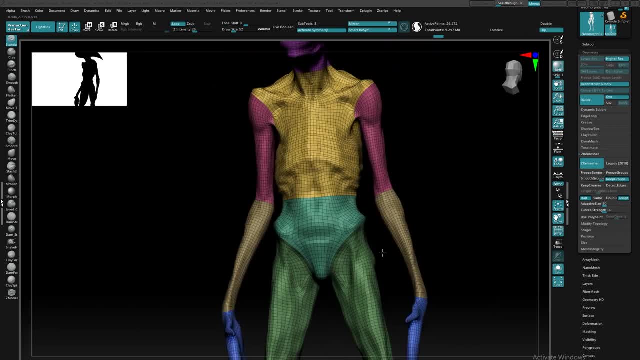 ease of use when manipulating my geometry. Now, once I have my new low poly, I want to make sure that my original dynamesh is turned down. So I'm going to hit Zremesh and then I'm going to hit Zremesh. 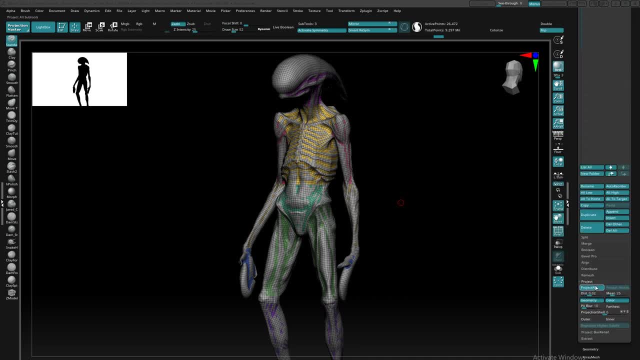 So I'm going to hit Zremesh and then I'm going to hit Zremesh On so that I can start re-projecting the detail back into this new low poly mesh. When re-projecting, I like to go level by level on each subdivision level. 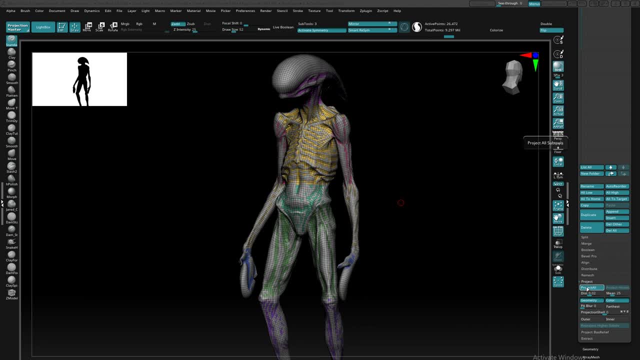 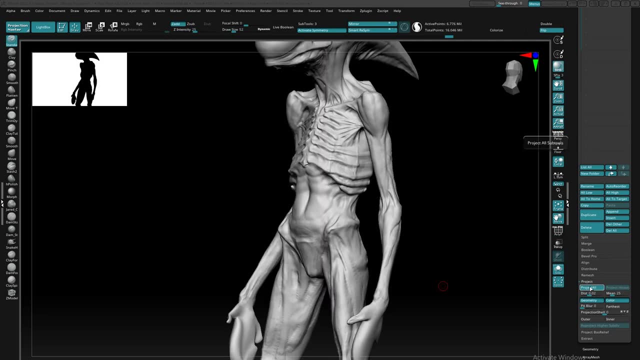 This usually just gives me a little bit of an easier time to make sure that none of my polygons snap to surfaces that they shouldn't, and it just gives me a little bit of a cleaner result. And just like that, now I have a nice quadded out mesh. I have polygroups for nice selections. 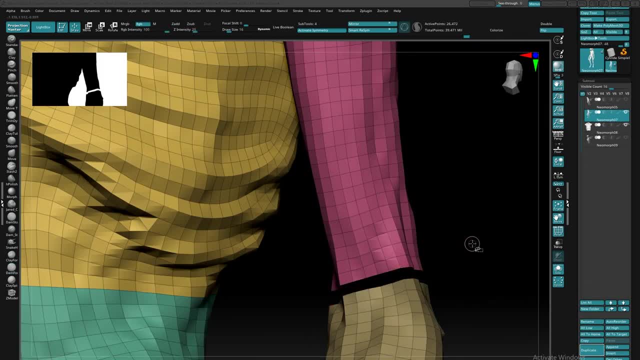 I have subdivisions so that I can refine my forms a little bit easier, and I have nice polygroups for nice selections. I have subdivisions so that I can refine my forms a little bit easier, and I have nice polygroups for nice selections. I have subdivisions so that I can refine my forms a little bit easier, and I have nice edge loops in a lot of different areas. 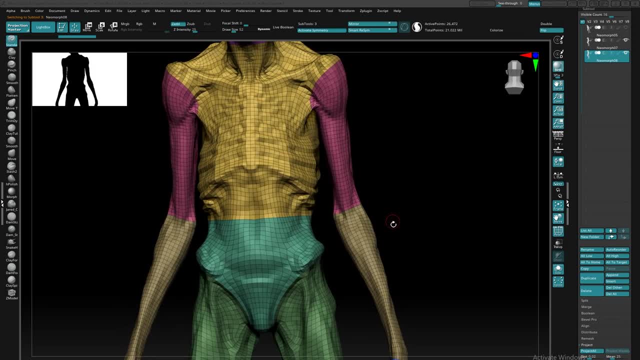 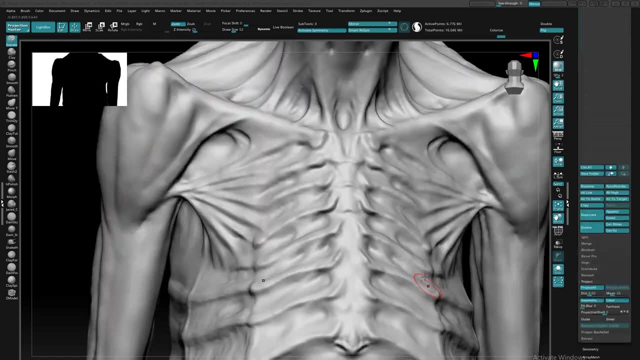 So if I wanted to call this good, I could continue to move on with my sculpt and refine further, which I will do, but at a certain point I'm going to get to the detailing stage of my model, And because this model is one contiguous mesh, that means that I will most likely only subdivide. 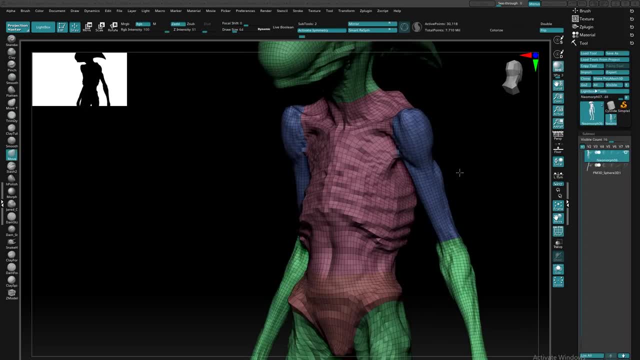 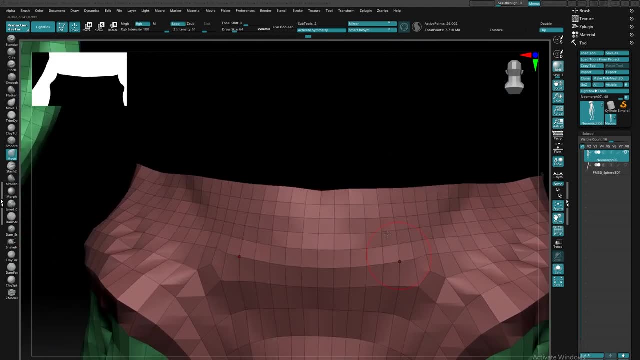